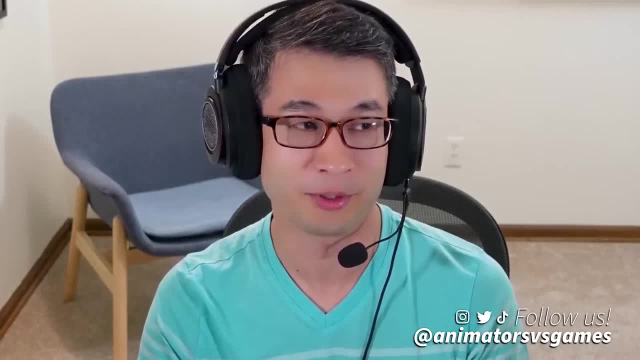 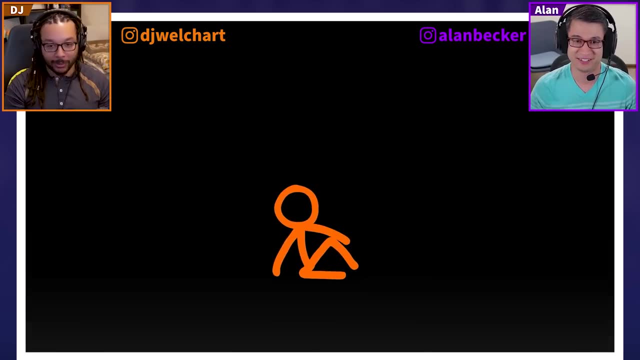 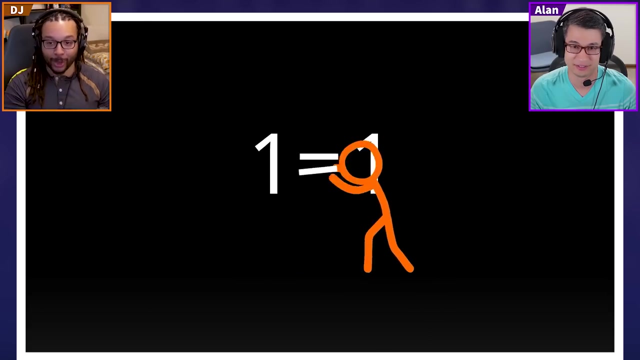 What up AVG crew Today? we are. well, I am showing DJ. animation versus math. I know nothing about this. No, he didn't even know the title. Ah, the number one, Yes, Where it all begins. Indeed, Oh, This is straight up math, Okay, Yeah, Oh, wow, Okay, It's straight up math. 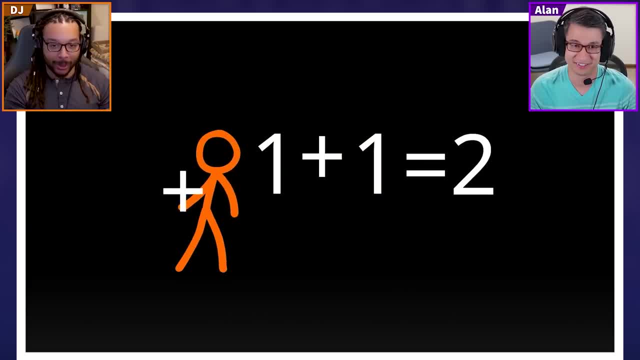 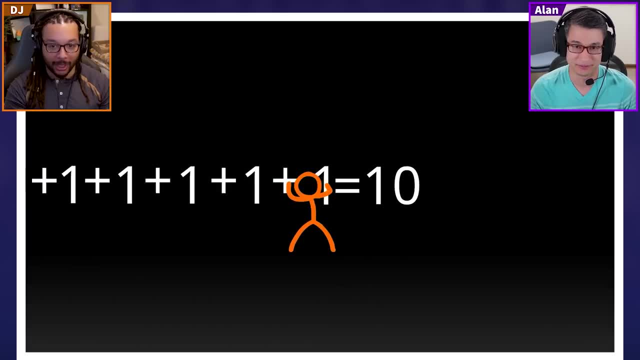 You like math, don't you? I do love math. That used to be like one of my big passions when I was a kid. Oh really, Yeah. How into math did you get I got into calculus by 10th grade. Oh my gosh, I didn't even do calculus, I got into pre-calc. 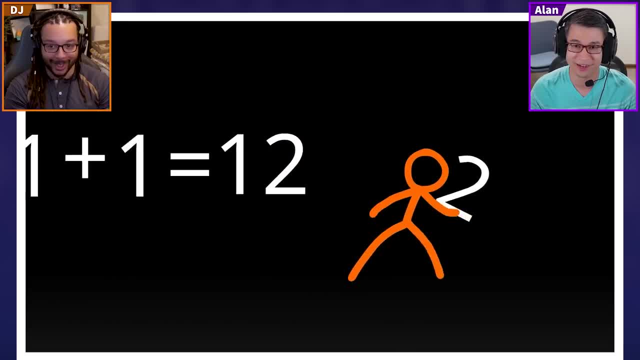 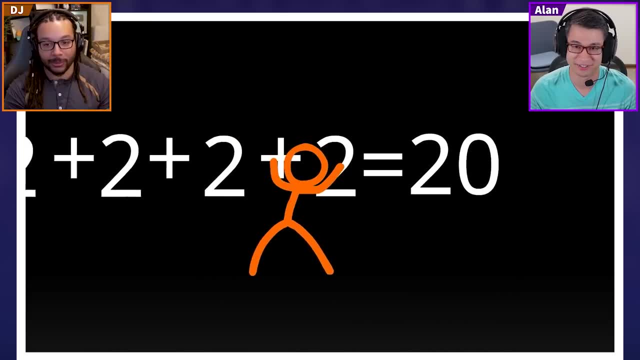 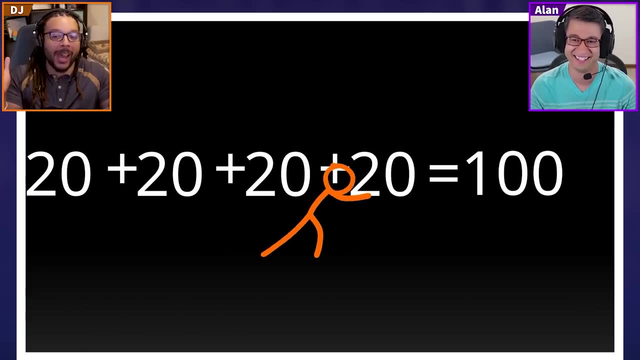 I would take math classes in the summer for funsies. so, Oh wow, I couldn't. I can't read and spell too well, but math I just understood. Max min. Yes, you know it, Dude, he's just, he's just like me with a kid. So much fun, Just math, guys. Oh my God. 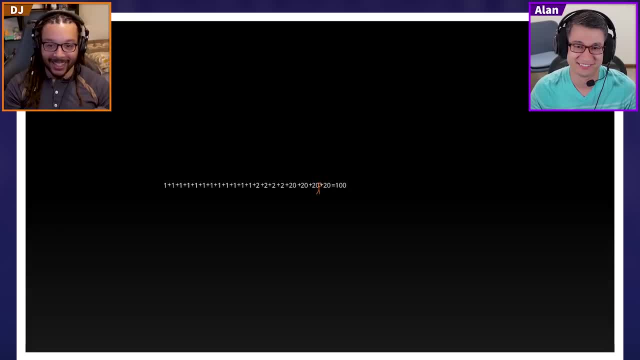 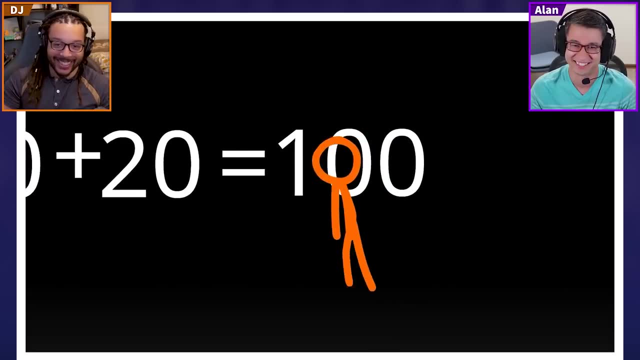 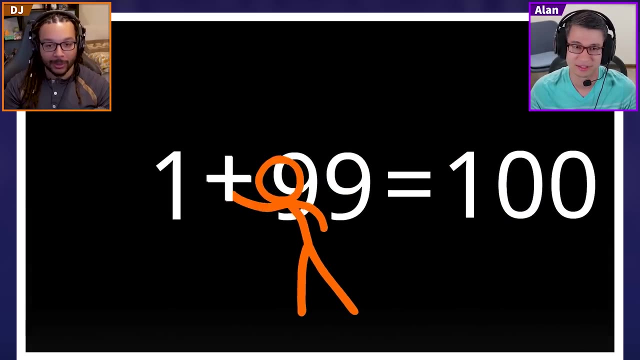 Math's so fun. He did it. Oh, 100.. Yay, That's the end of the numbers. It's the highest one. Yeah, Oh, Ooh, Go keep that. Yeah, that's good, Yeah, that's good. 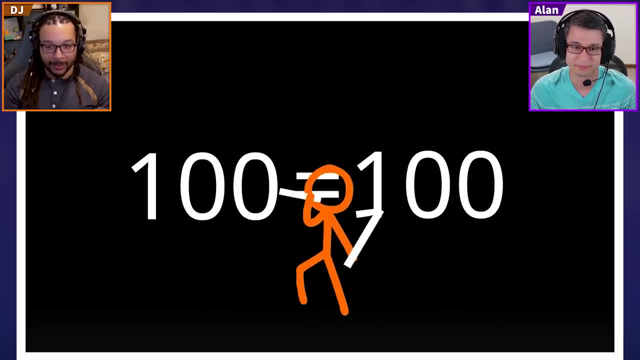 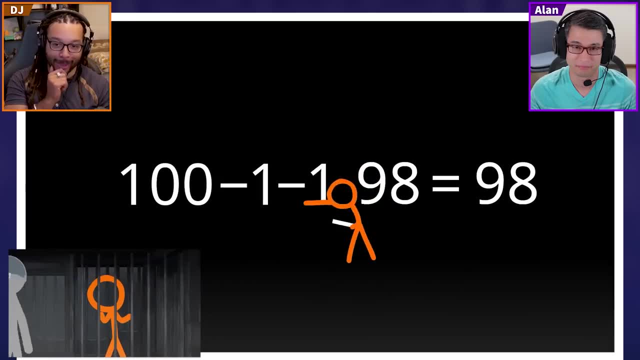 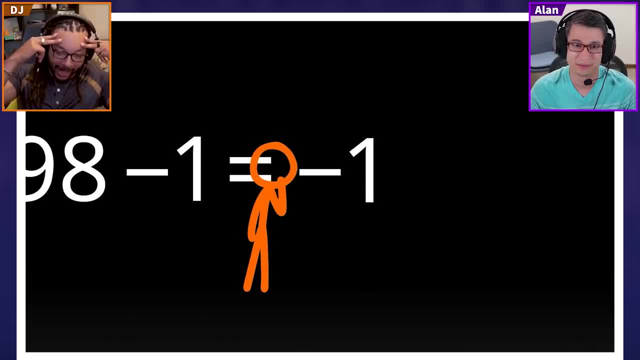 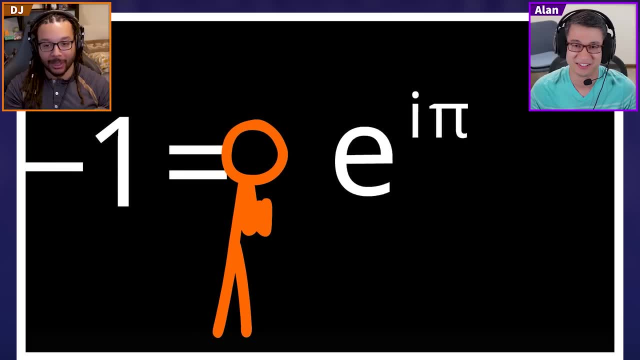 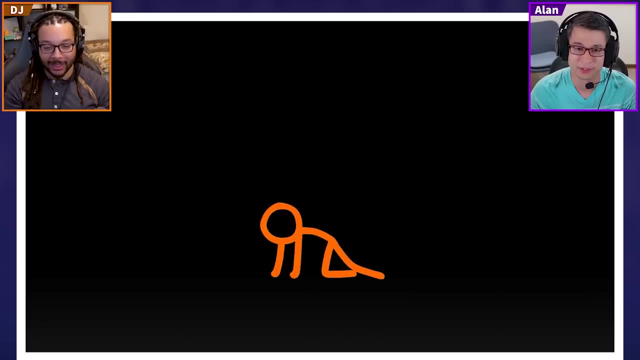 Yeah, Oh yeah, I see He's bored. He's like I gotta do math. You know what that is? Uh, I didn't know what it was either. I didn't actually come up with the story of this, It was one. 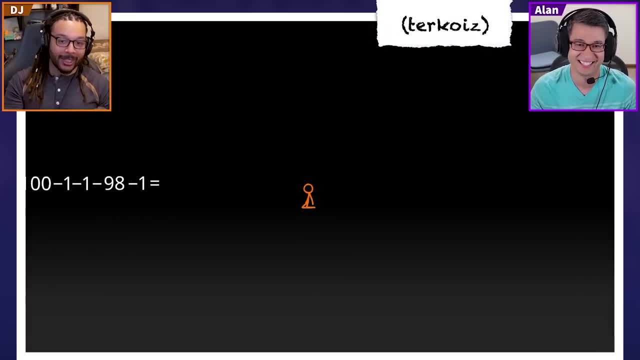 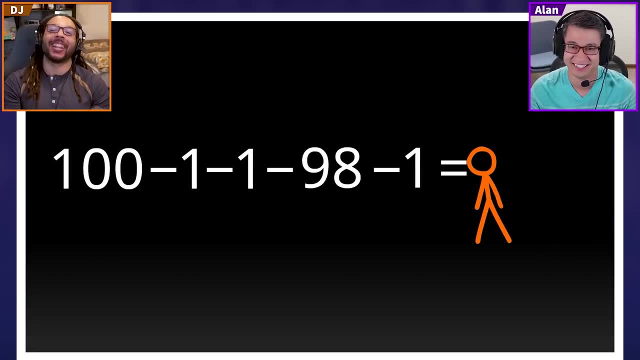 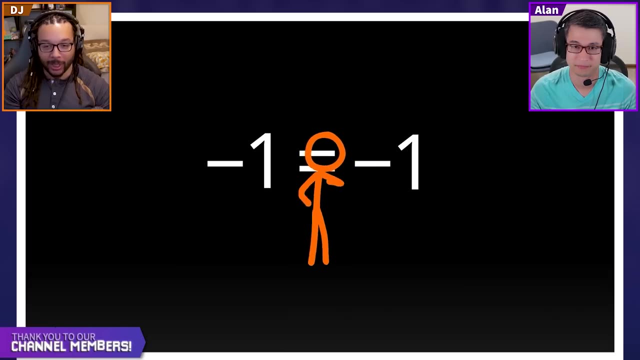 It was one of my lead animators, Math Dang it Pie. I was going to eat it, So hungry. Yeah, that's totally what he was thinking. Just looks up in the sky like, oh, Hmm, Wow, Everything equals one, and now it equals negative one. 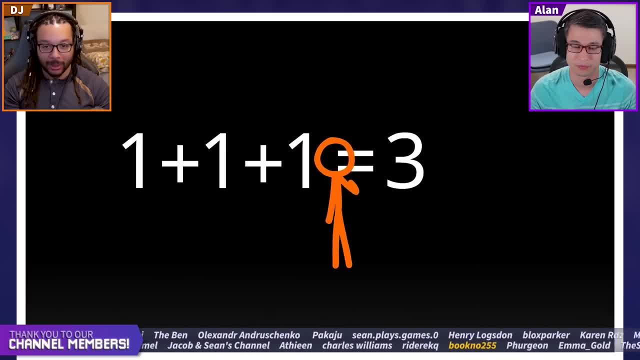 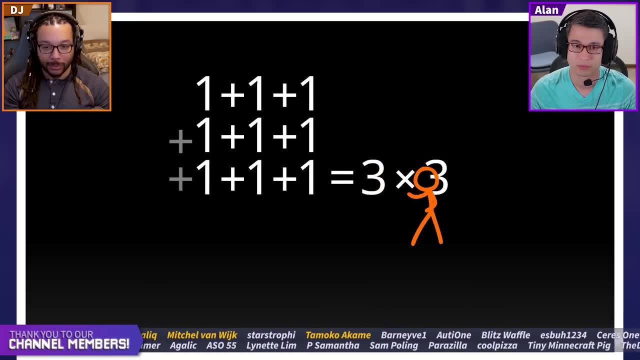 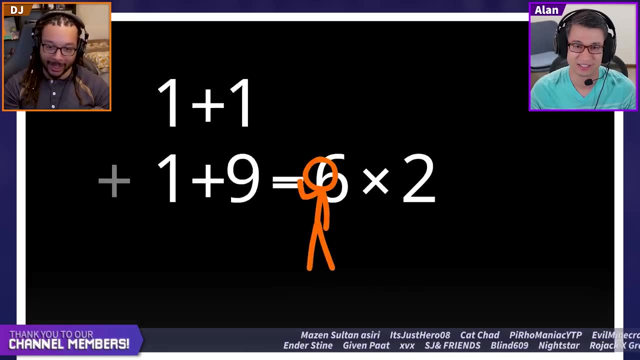 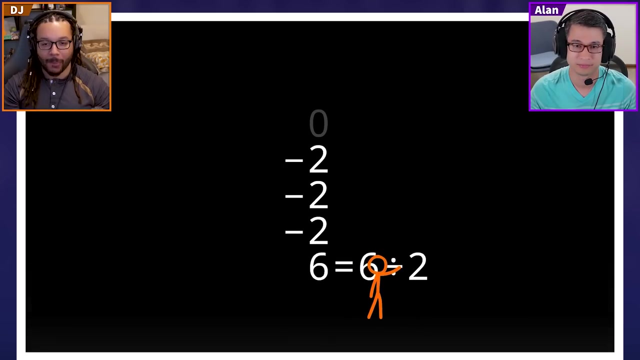 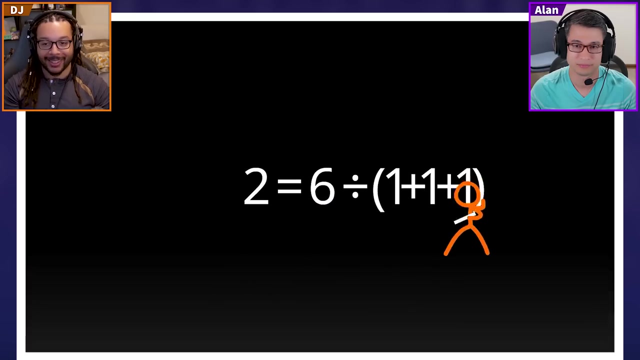 And now it equals negative three. Oh interesting, Oh nice dude. Math would be even more fun if it was, uh, like this. This is great. Yeah, Yeah, Huh. That's cool dude. I want a calculator like this. 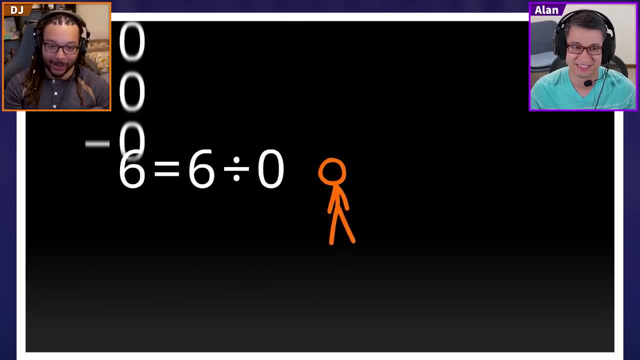 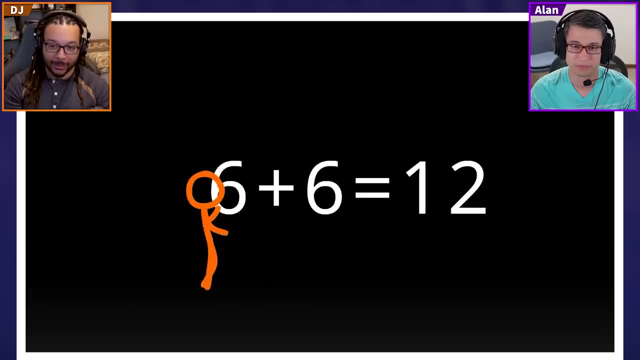 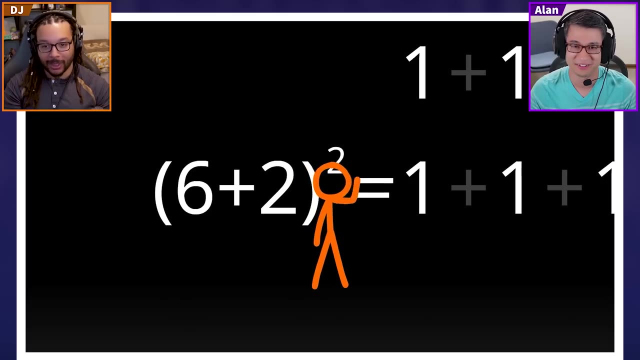 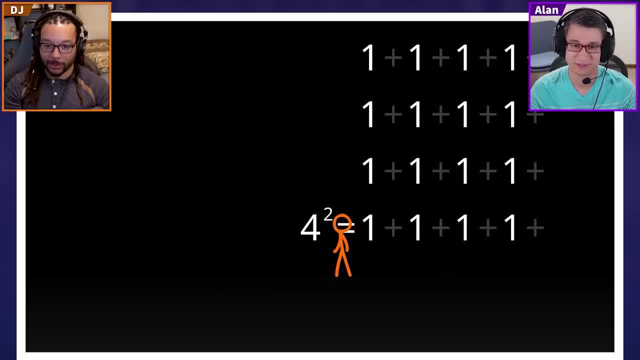 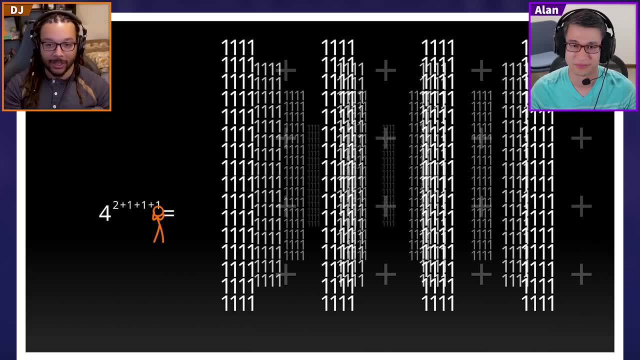 So he just has to figure it all out. Yeah, He's a fast learner. They're, they're, I. I still stand by like their super power is all like super elasticity, brain power. It's like a child smarter right. 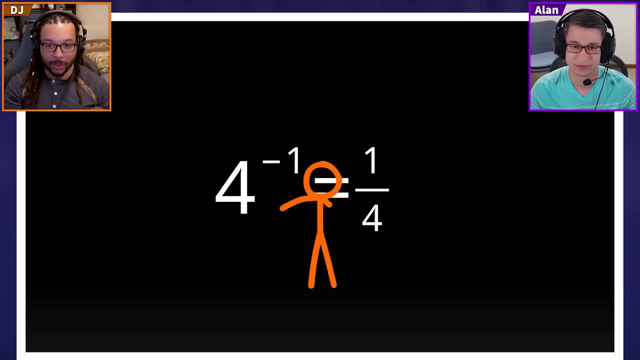 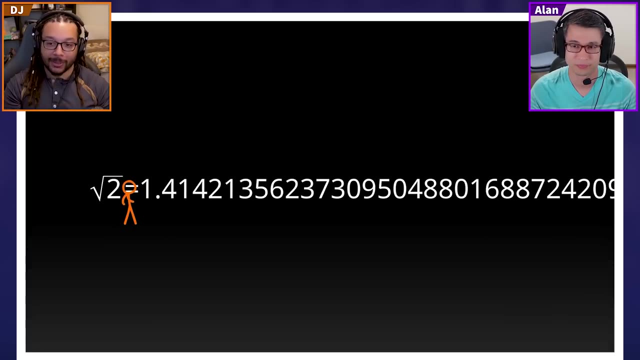 It's like as we get older, we just get worse and worse at like, understanding new concepts and stuff. Yeah, Kids and your stick figures. We just learn so fast. The neurons are very rigid. They're all neurons. He's going through everything. 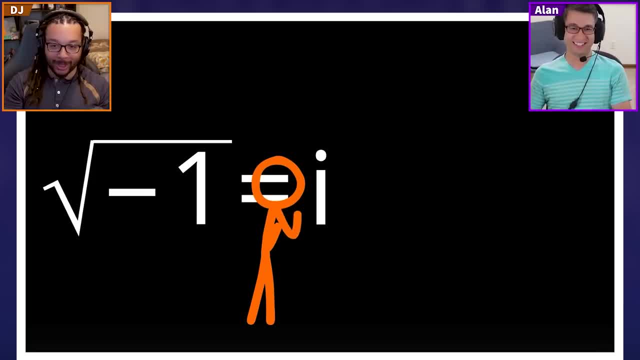 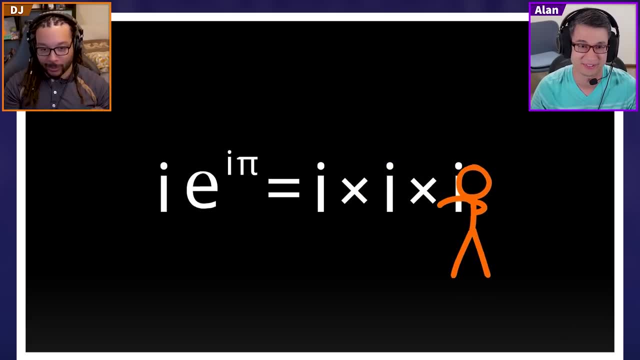 What about the door that took the number? What, what, what was the number that he took? That was Oilers number, Oilers. I don't remember any of that. No, I didn't learn it either. Is it like Calc, BC or something? 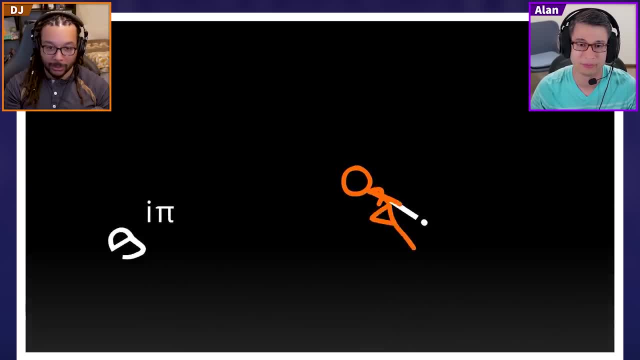 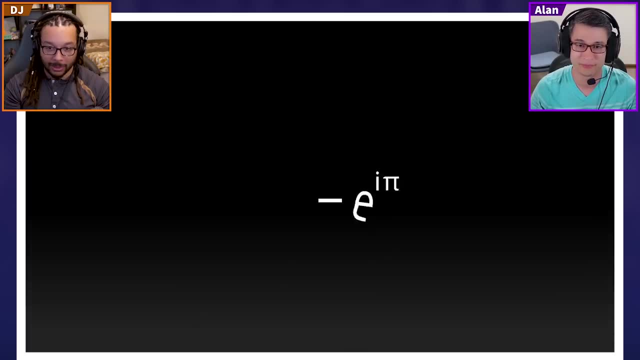 Um, I think I don't want to. So like my, my lead animator came up with the whole story for this cause he's a big math nerd. Um, yeah, he, he's a real math nerd. I'm a fake one. 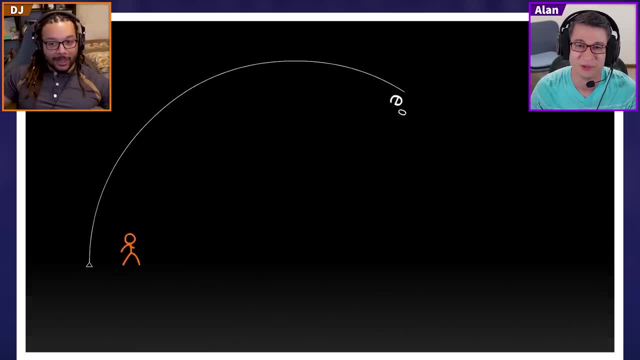 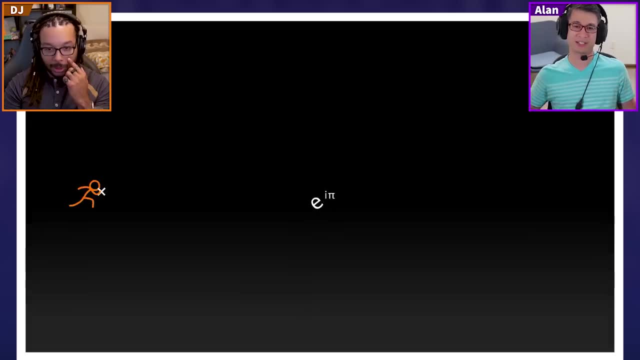 Yeah, I don't remember anything. I don't even know if you learn about Oilers number in school, but it's supposed to like encompass all of like math or something, All imaginary numbers or something, And it also equals negative one at the end of the day. 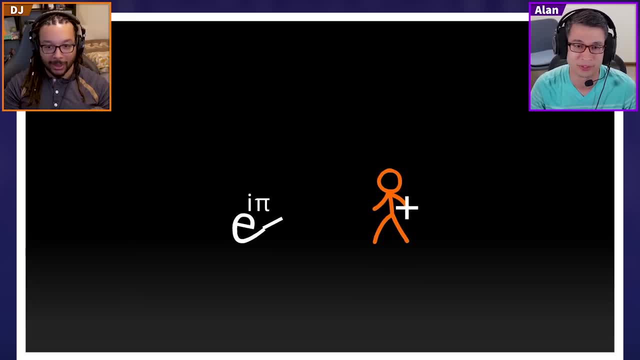 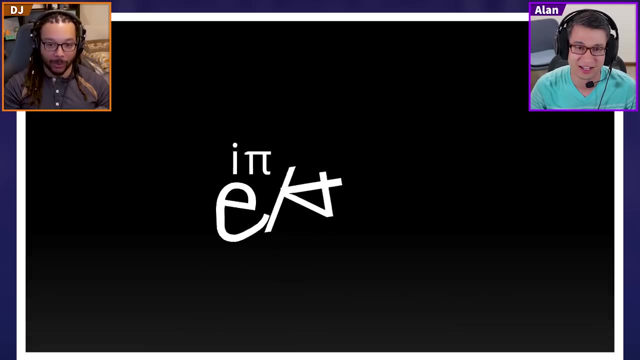 So that's why when he poked negative one, it became Oilers number. He has a plus when he was holding it like a cross. Yeah, yeah, yeah, Back higher. How many uh communions do you need to take before you've eaten one Jesus? 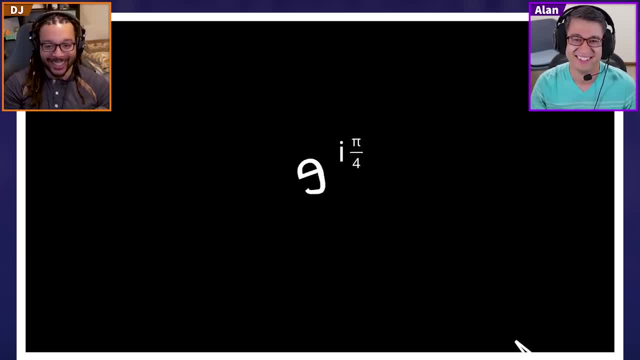 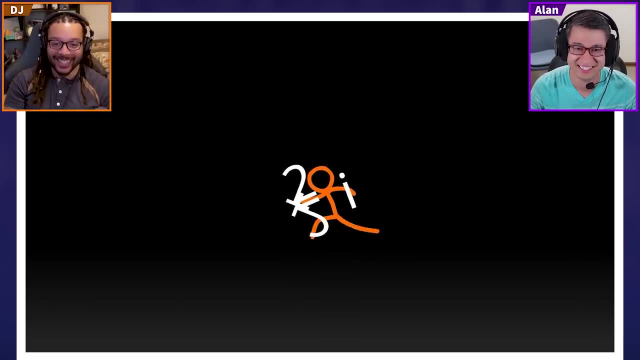 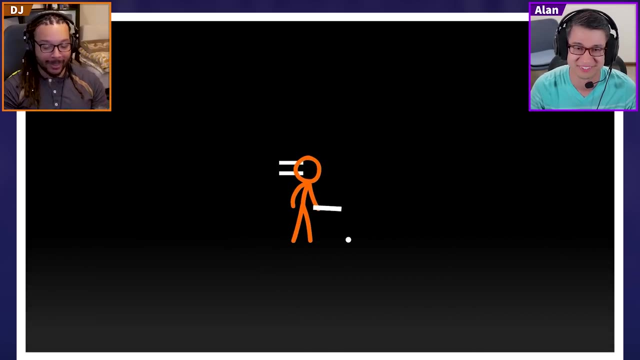 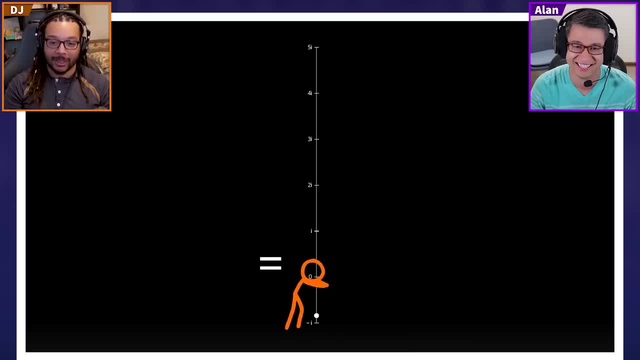 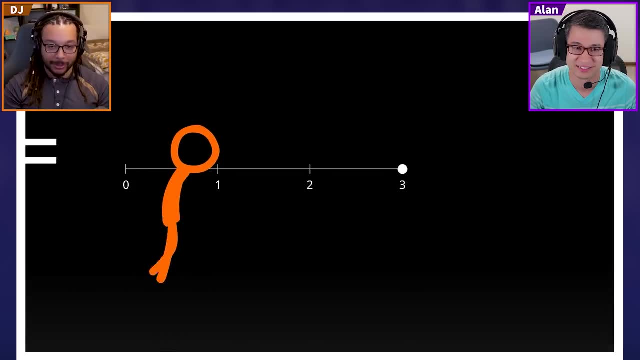 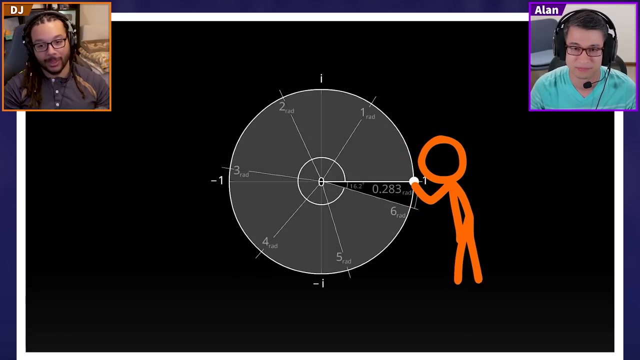 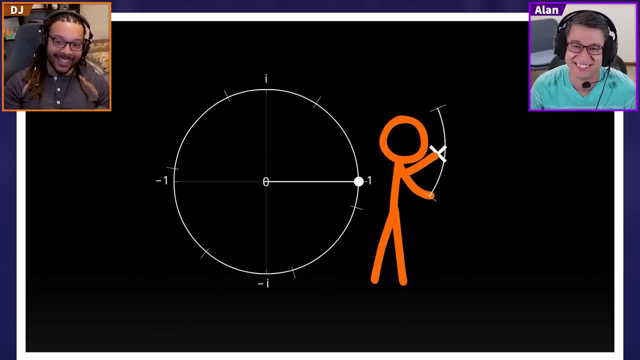 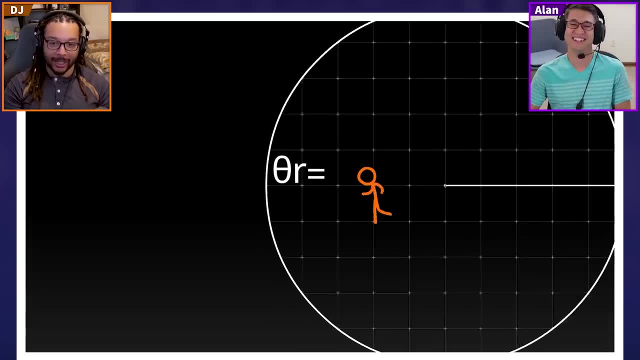 He's just: No, you don't, You never see anyone else. Dude, I'm going to say this one, This one is- I'm putting this in the lore- He's in jail, He's sitting there and he's just like bored in his head playing with math. 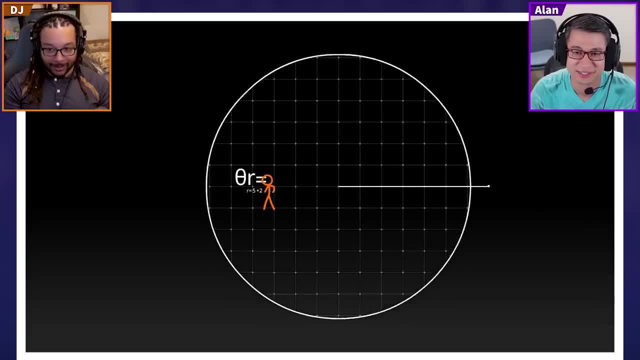 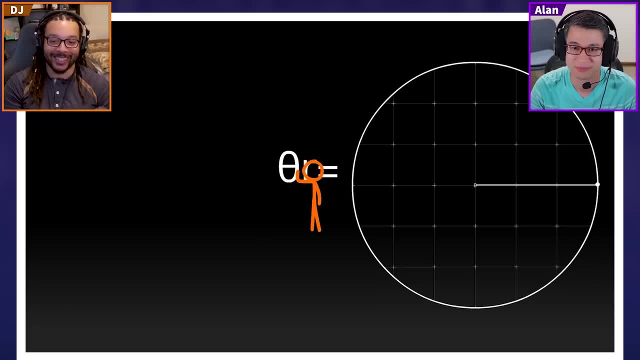 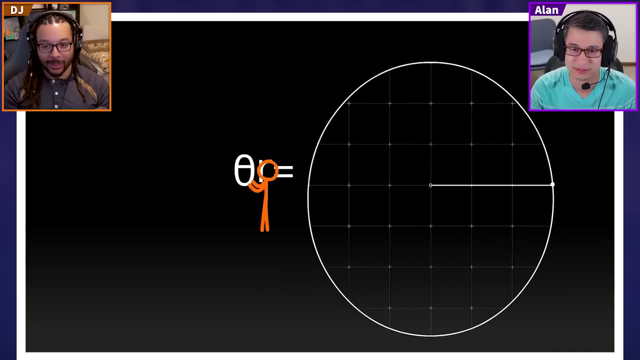 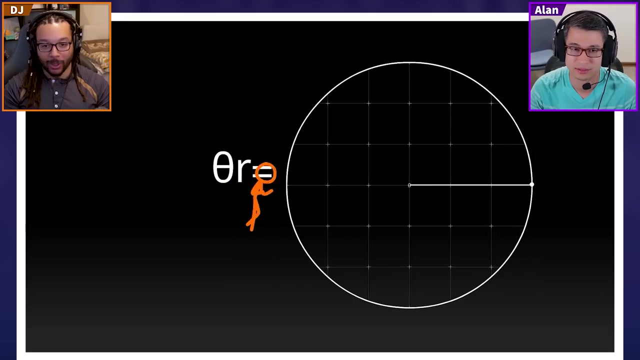 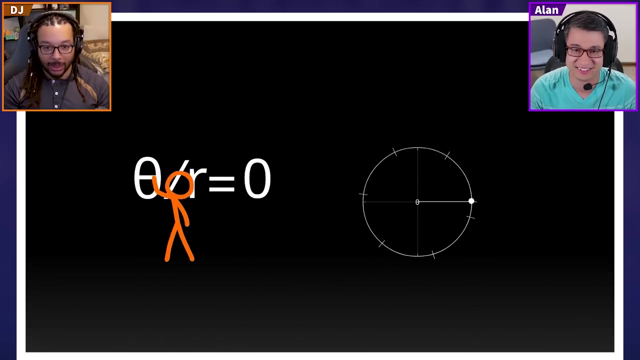 Yeah, Okay, When he comes, when he gets out of jail, he's going to fight with the power of numbers. Yeah, This is like, just like going through, like all of high school in a video. What math did you get to? 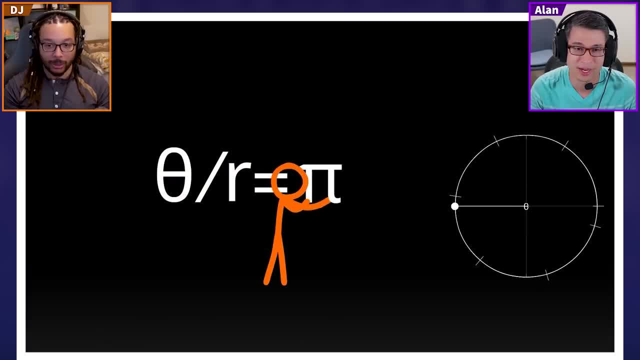 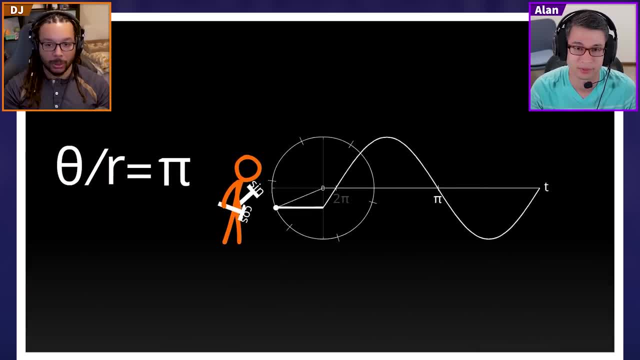 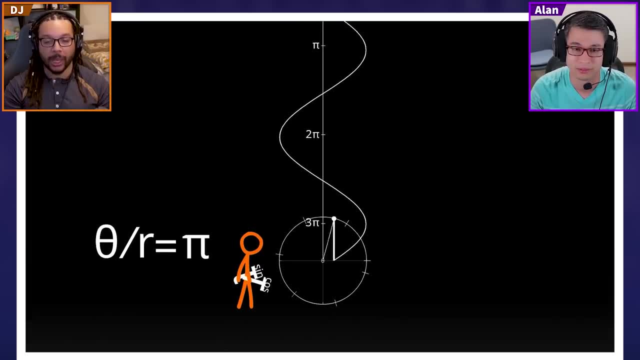 Okay, Trigonometry: Yeah, I know what trigonometry is, but I don't know, So I'm going to just ask, because of my school, precalc and trig were one class. Oh, really, Okay, Yeah, Well, I don't think. they said it was trig. 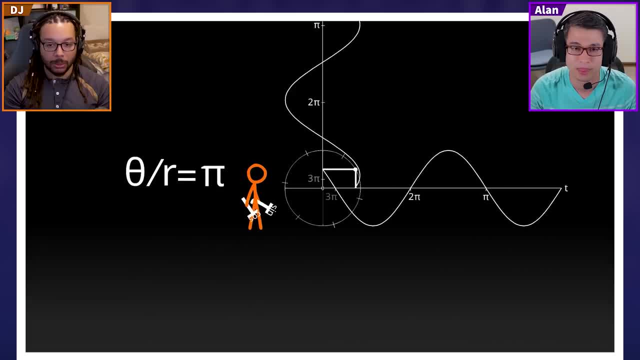 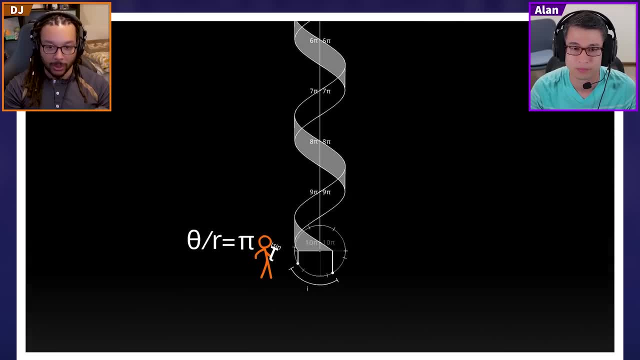 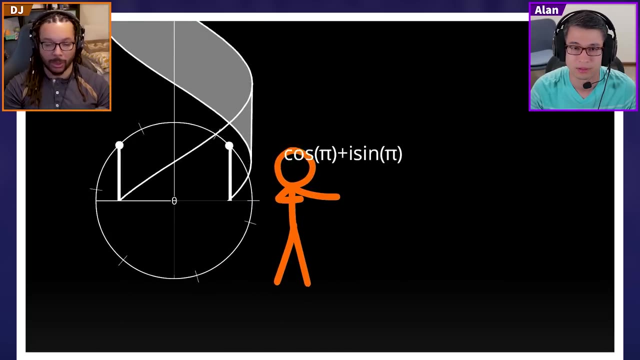 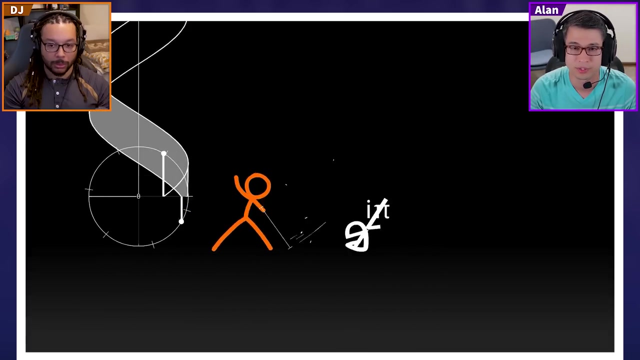 Okay, I mean some people end high school in like just statistics or even geometry, Right right right. I had friends who never got past geometry Or even algebra two or something. Yeah, it was mostly because my school before high school didn't start me early with algebra. 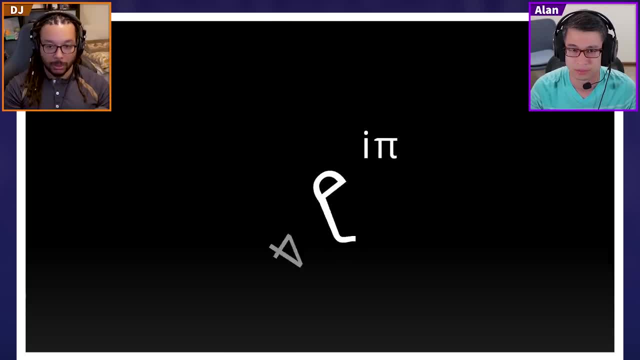 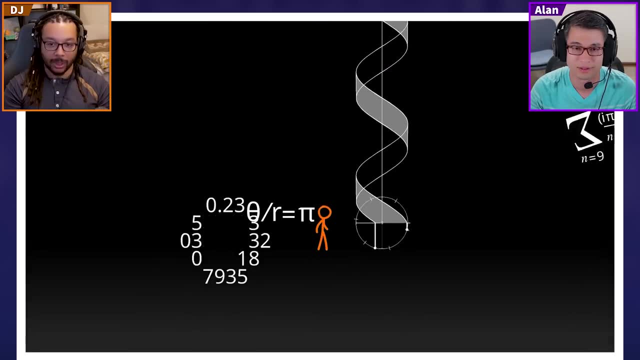 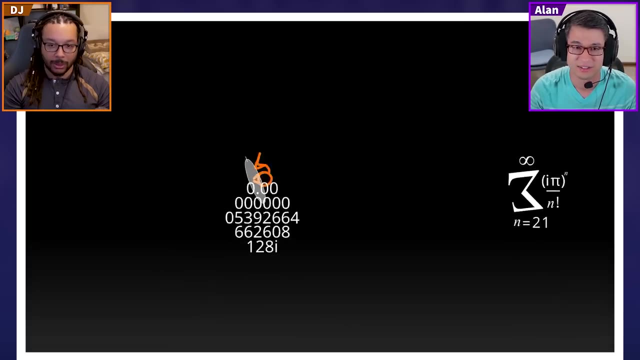 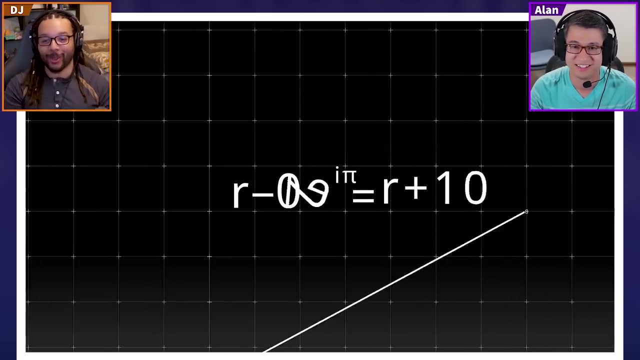 So I was behind here? Yeah, I don't think. in my high school, if you were in trig in that class, I don't think you'd still been ahead of most of my friends. Yeah, Yeah, Yeah, Yeah, Dude, everyone's just doing math. 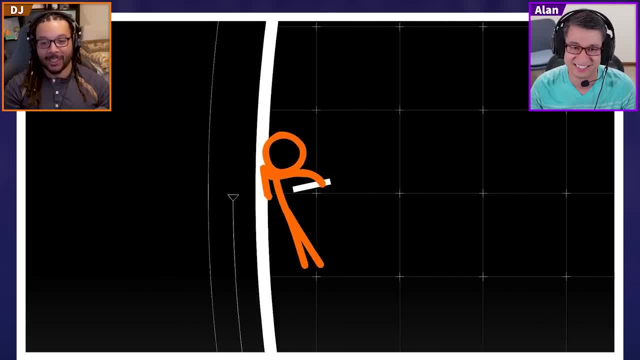 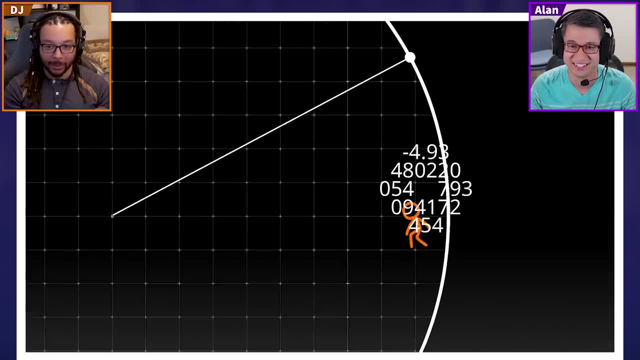 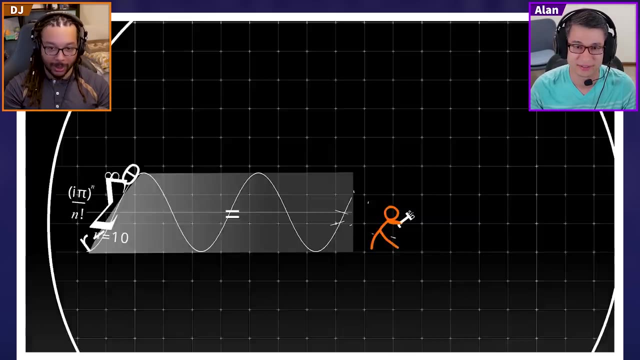 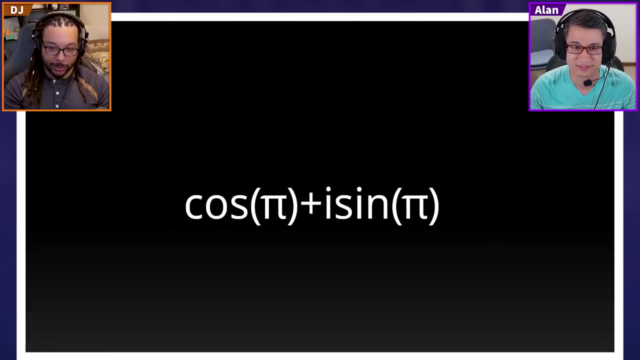 is going so hard. Oh, Pac-Man, Okay, Pac-Man, strat, Go the opposite way, Come out the other side. Oh Yeah, It's the minus sign, uh-huh, oh, is that a wave? yeah, um cosine wave. yeah, hey, oh no. 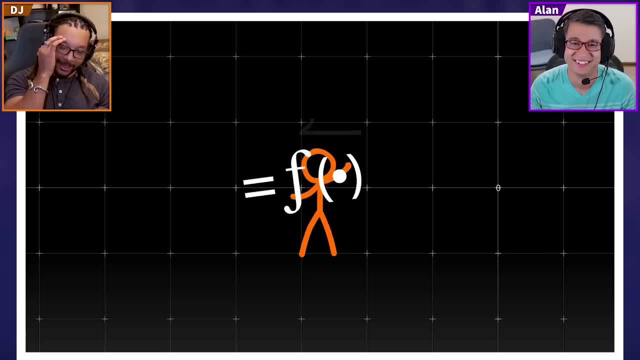 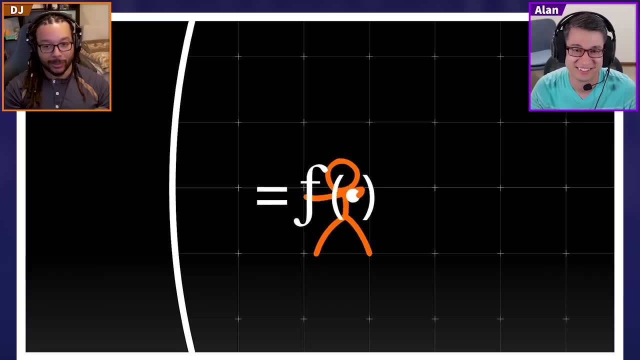 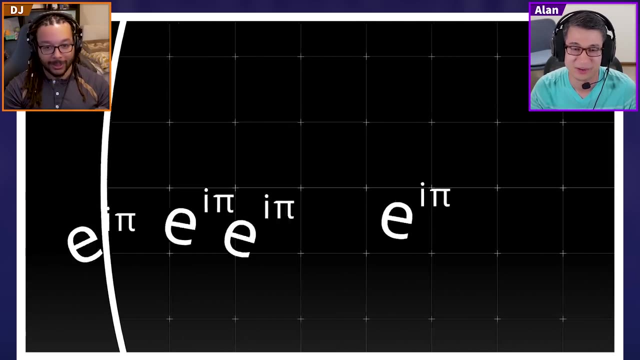 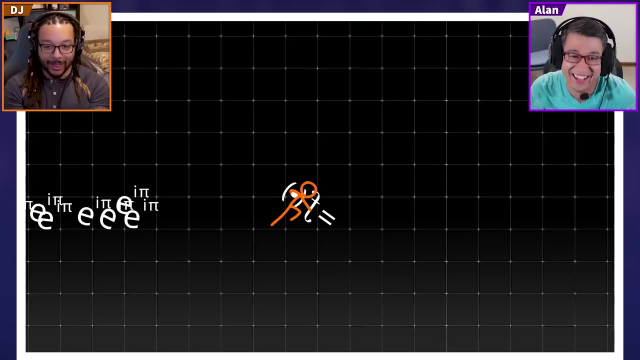 tangent- i don't even remember anything about those i know- and the co-tangent and the coast. oh yeah, it started getting crazy. yeah, get them. yeah, we don't expect like 99 of people to understand all the math in this dude, we don't even. i know you made this. 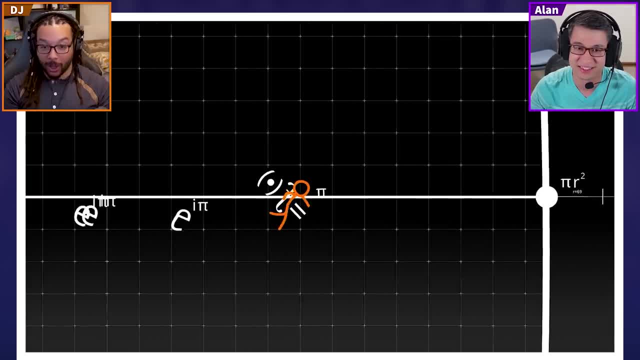 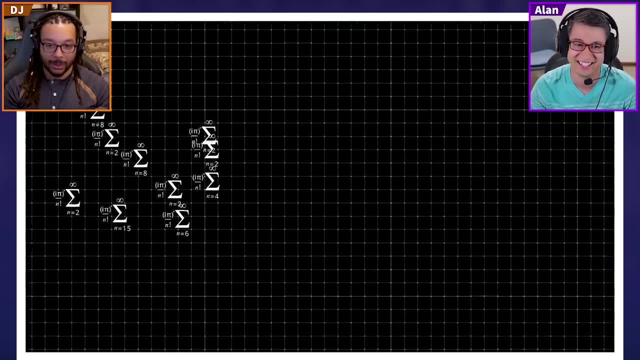 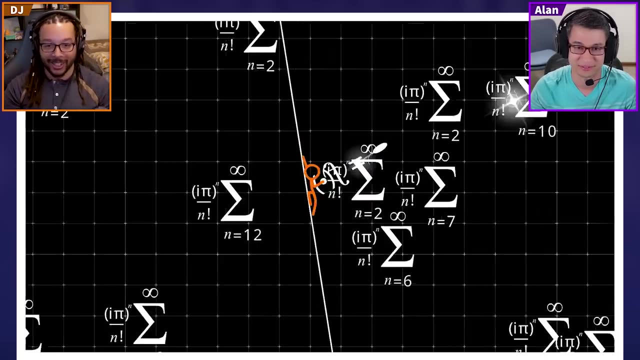 yeah, if anyone, if anyone understands all of this and who isn't a math major? uh, please let us know in the comments. yeah, i did show this to a math major and, uh, we understood all of it. was he like? i get it, was there a lot of that? uh, well, you know, i mean he was. uh, i feel like 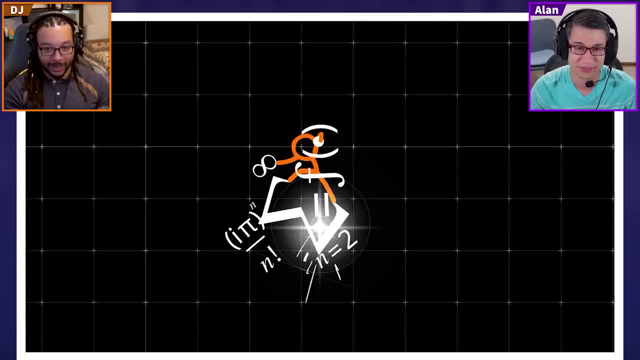 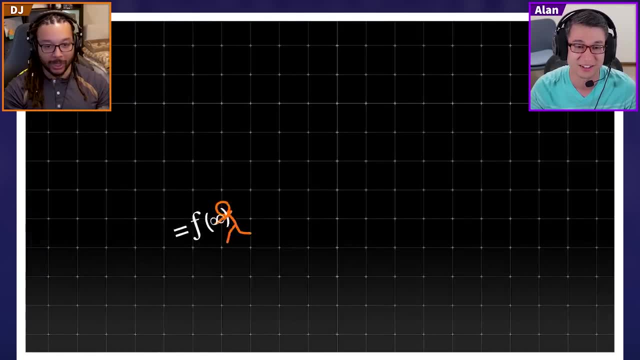 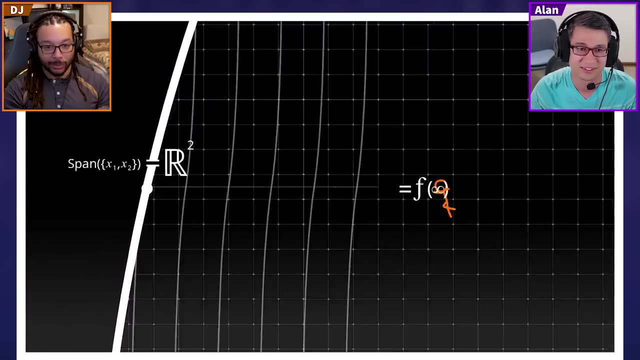 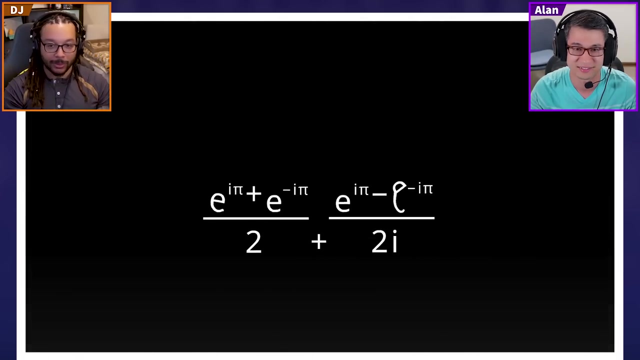 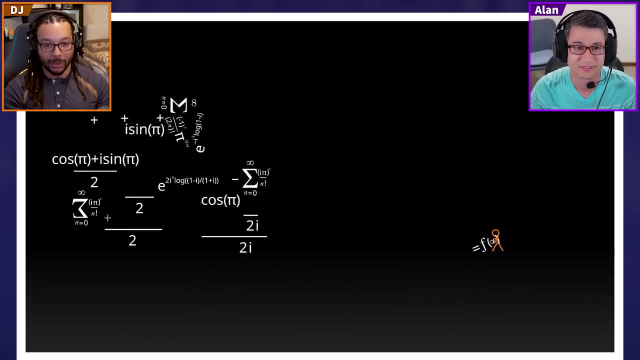 a lot of math majors are also pretty like i don't know, not emotional. so, yeah, like blank-faced infinity, you can tell that he appreciated it. nice, yeah, you better run, got the infinity gun. this is so cool. they just could kind of like run and do math. that's so neat. 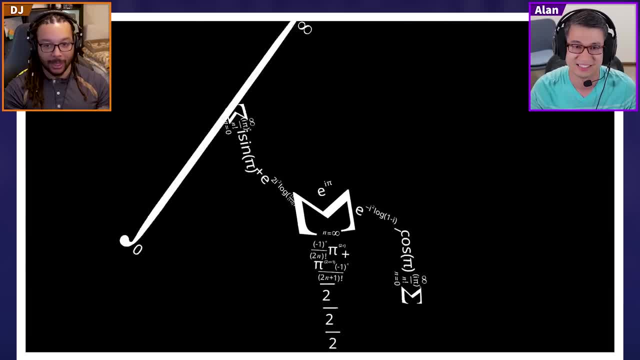 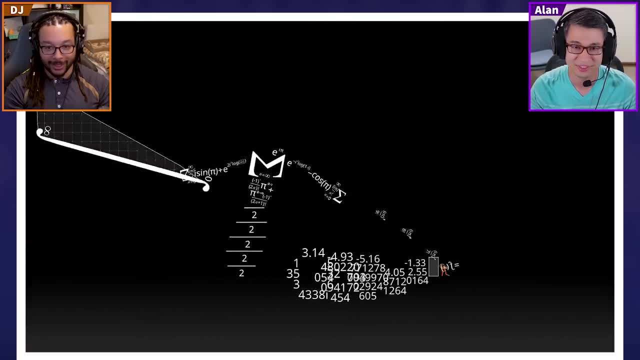 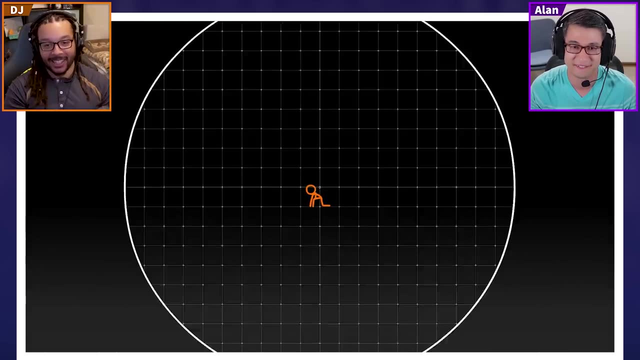 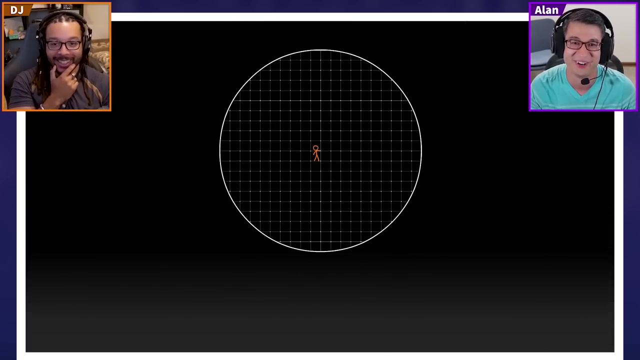 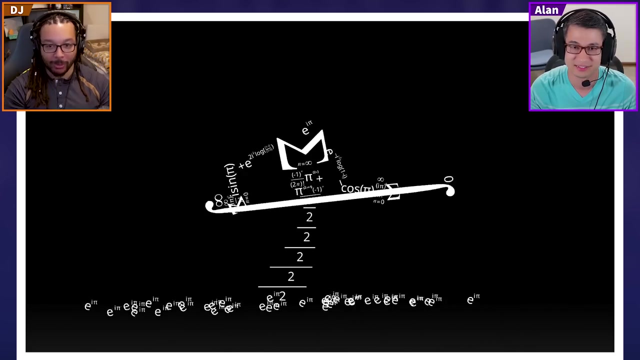 yes, gundam, he's got all of the numbers. geez, the dark souls boss here. like when you walk up to the boss and then you just see the health bar show up at the top like oh no, oh no, health bar. okay, i have to fight him. oh god, he knows math. now he's awake. oh cool, he's just climbing. 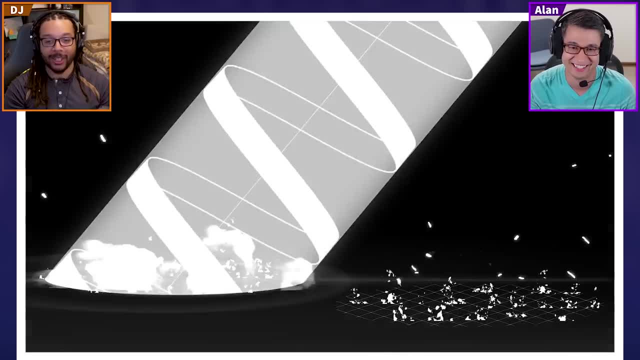 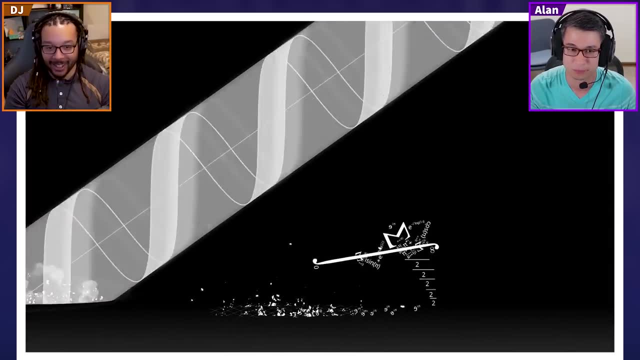 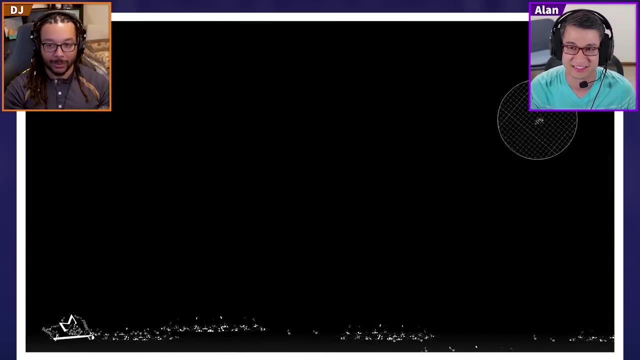 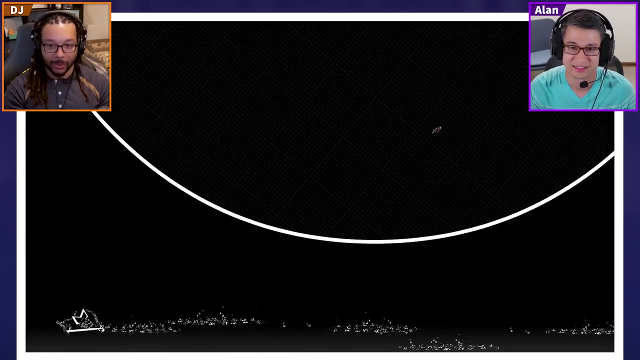 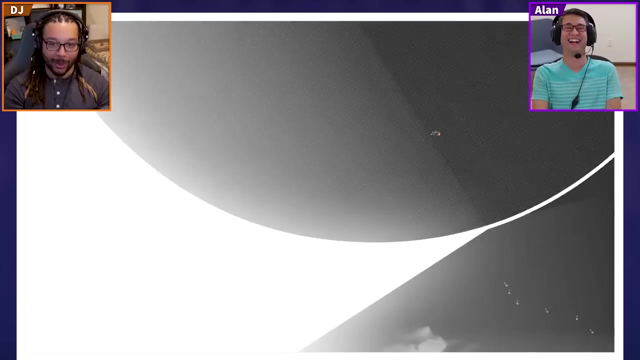 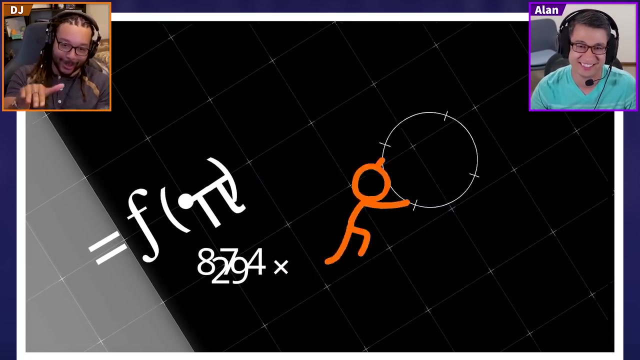 oh, that was sick. how are you making math so cool? yeah, oh man, what you gotta do now reloaded? oh my god, jesus, you don't need to aim it at that point. dude like, why are you sure you get it on right on the target, you want to make sure it does maximum crit damage, like 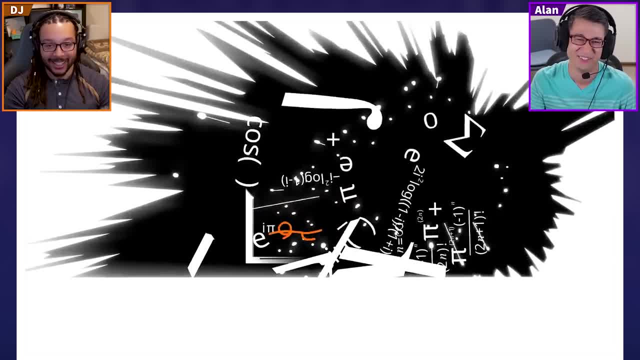 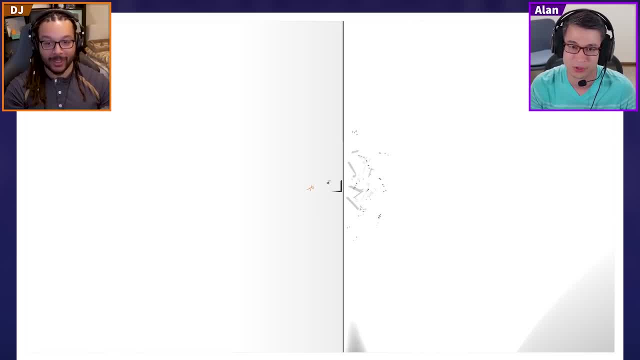 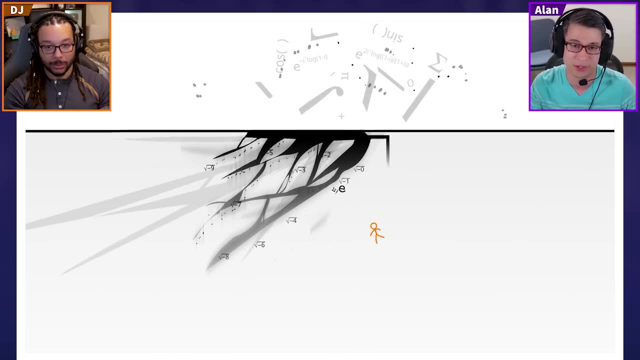 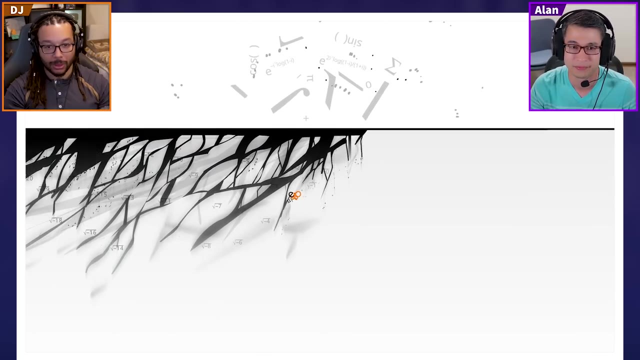 run, run negative one. run negative one. is that your name for him now? no, oh so all of this is supposed to be mathematically accurate. when he multiplies himself by i, he goes into another dimension and it's 90 degrees rotated. interesting. it's like when you joke around and divide by zero, or something like that when you're a kid. 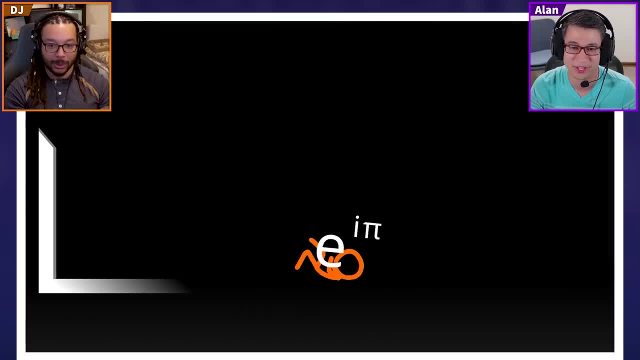 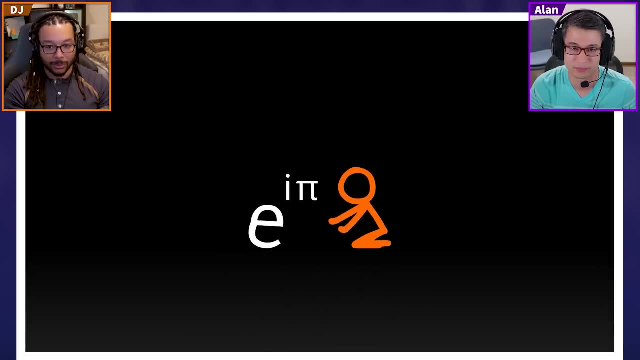 right, but more math, but more factual, more than that. yeah, hey, i don't want to have to kill anymore. i've killed so many more people. i'm a little scared and some of you can't, hey, hey, i'm also a little scared. i hope you don't get that. 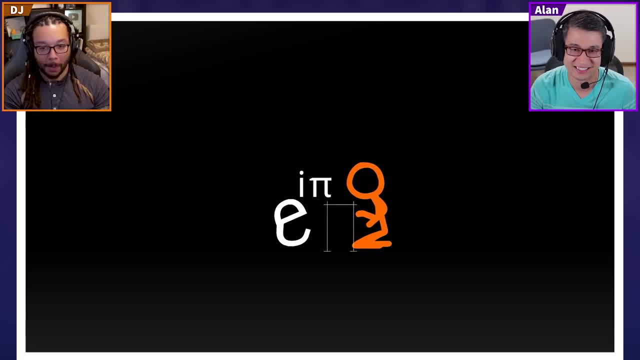 oh, you've been picking up from us, yeah, and we're going to have to do our own, and then i'll just go in here and i'll just do my own, and then i'll just go into the other world and can't do that, and i'm going to go into the other world. 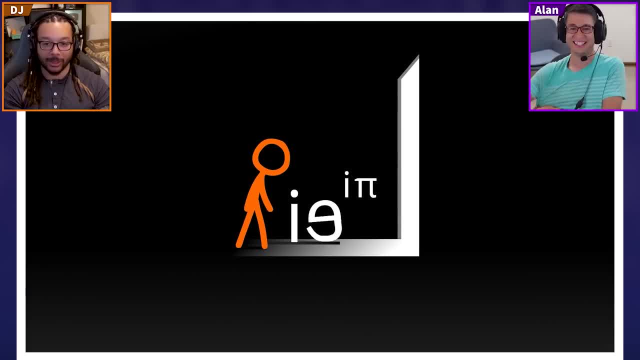 i have to do that, but what i need to do is to make sure that i'm not going to get hit by a libro. so if you go to the other world and then you go out into this world, you just kind of get picked up by that, like you had to go in and do everything else in that way. 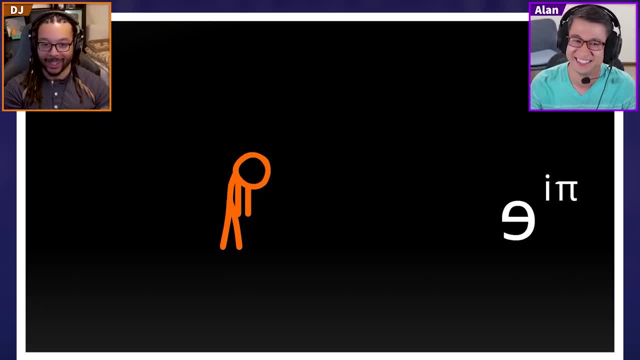 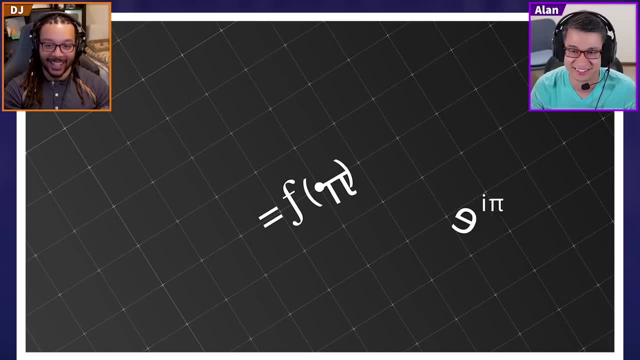 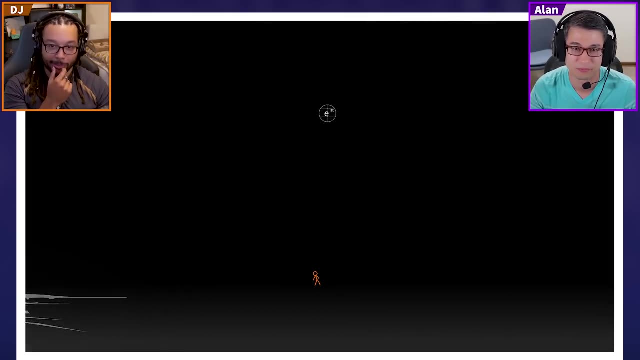 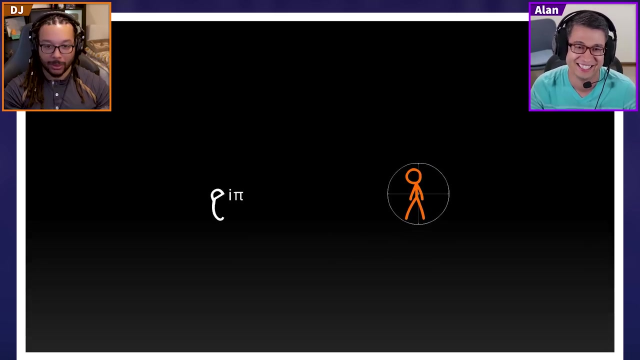 My brain's trying to understand any number math equations I can kind of get. I can't go into like words: Shoot, That's good. Goodbye, Get in the elevator. Is the um? does the E live on your computer? 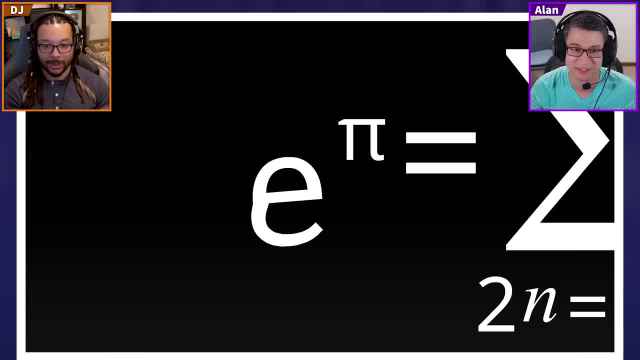 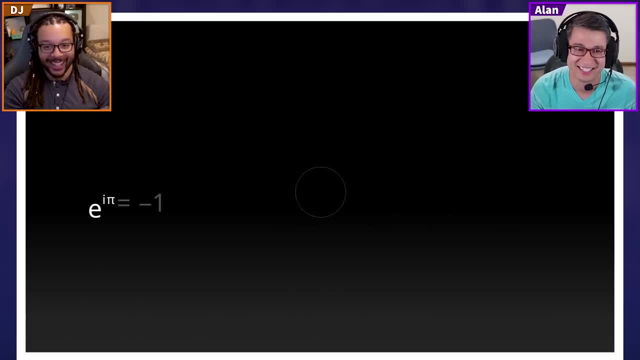 Now, Oh, I mean, I'm not answering that. Okay, Could be a reoccurring character of math. He is math. Bye, Thanks, math. I'd like to see a like a math major react to this. 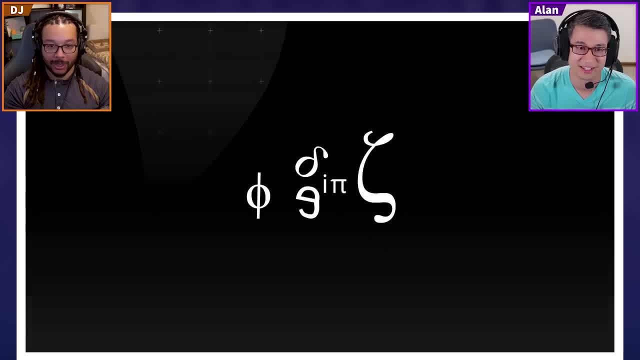 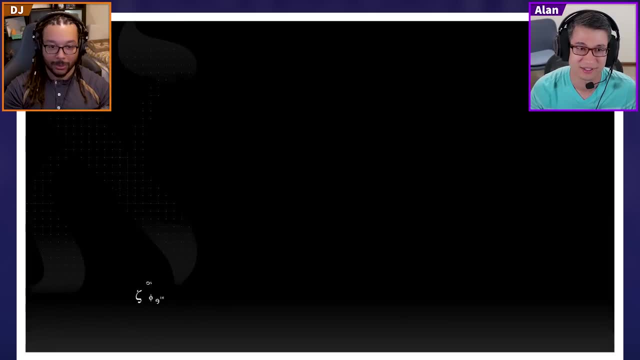 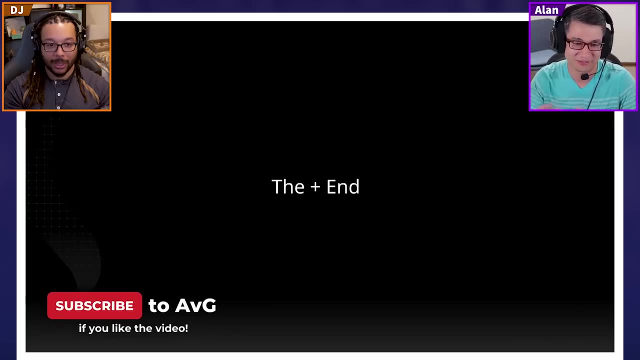 Me too, And explain what's going on. I mean, he told me you know most of everything. but Yeah, Apparently What? What is the giant? What is that It like encompasses all of you know something. 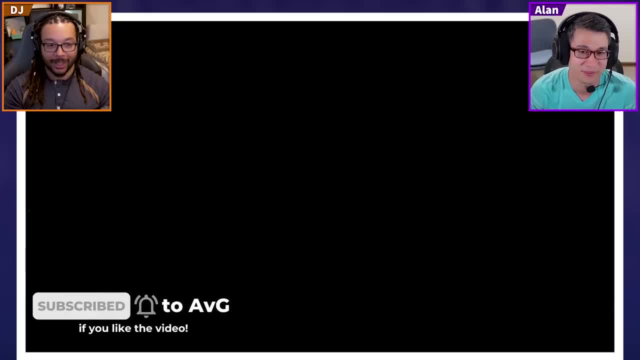 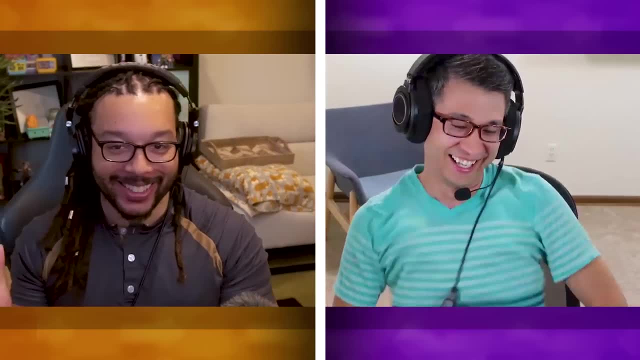 All of the numbers. I don't want to butcher the math, but The math of it. Yeah. What was the big, scary, ominous graph in the background? They were all math constants. I think This one was really interesting. 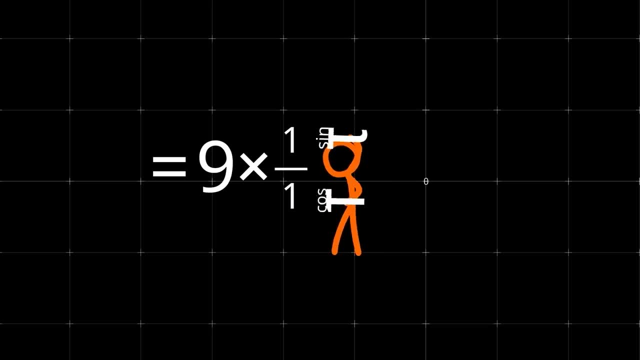 I've always wanted to tell a story with numbers like this. I'm definitely going to watch it a few more times and see what I can get out of it. Because it's funny, because you start off with such a basic concept in addition and then 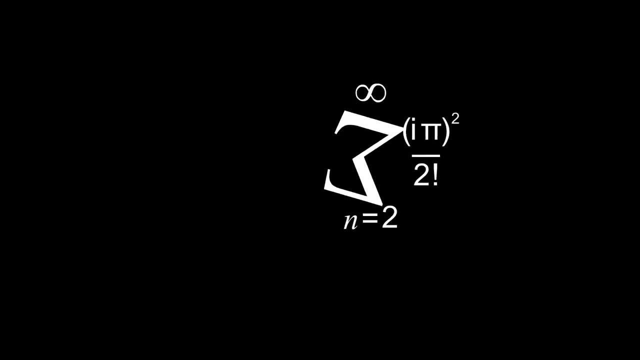 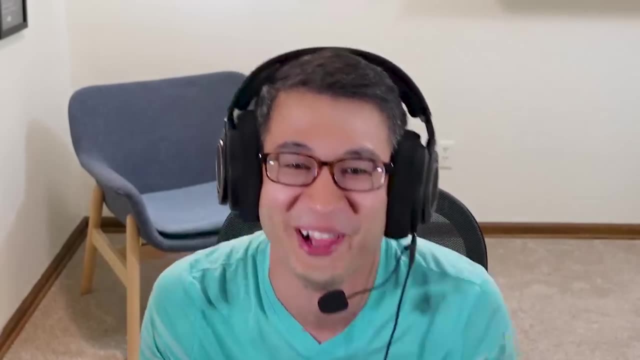 move into like such so much further than I ever got in math. I think It's interesting to when you fall off Right, Which everyone probably will. Yeah, yeah, You put it in the comments. When did you fall off?